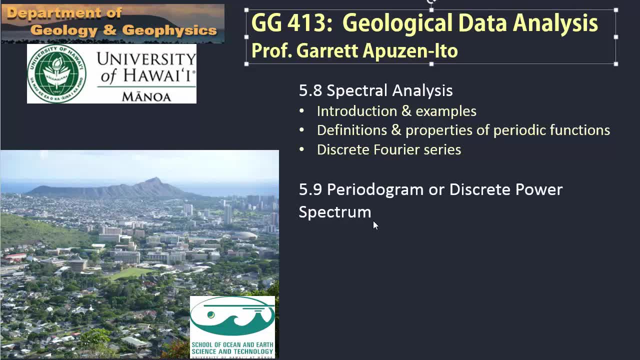 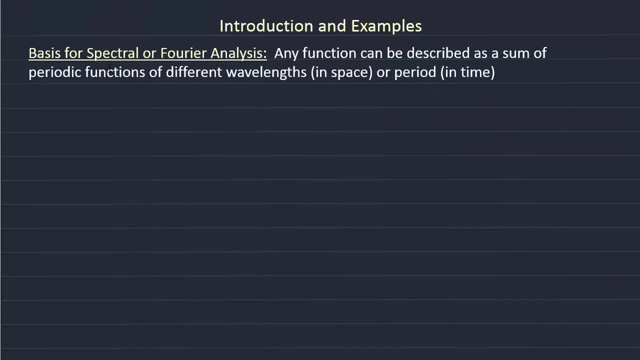 It's a way of identifying any key frequencies in your data sequence. So, starting on with introduction and examples, again, the basis for spectral or Fourier analysis is that any function can be described as a sum of periodic functions of different wavelengths, that is, if the sequence is a sequence in space. 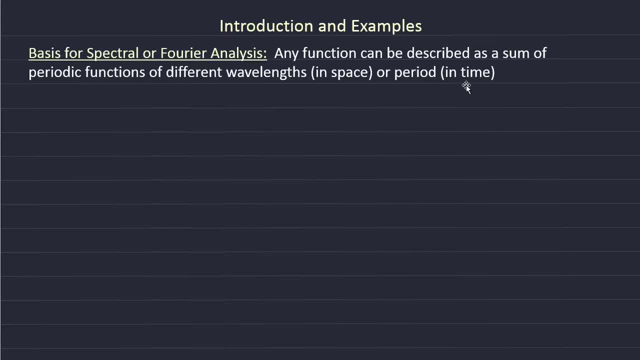 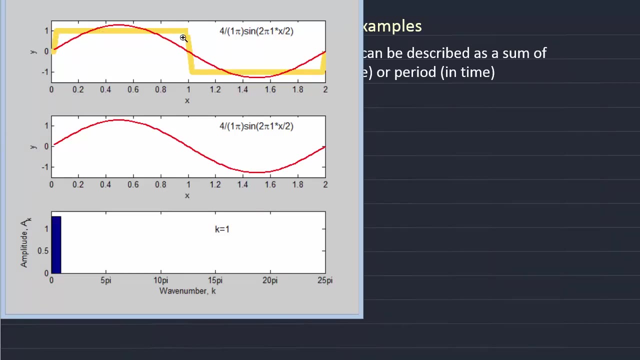 or any periodic functions of different periods, if it's a sequence in time. So my example here is a square wave. So this, the yellow, yellow curve, is an approximation to a square wave And the first component that makes up that square wave. 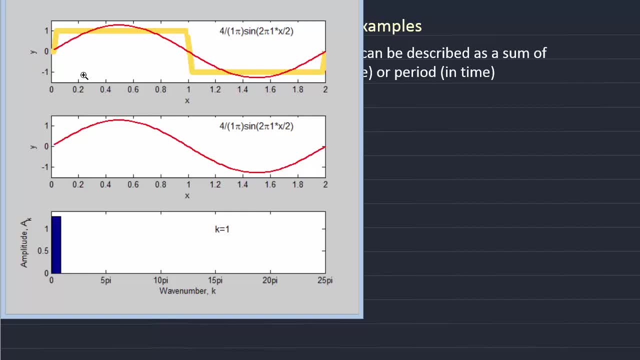 is a sine function with the wavelength of the whole data sequence going from x equals 0 to 2.. Now the bottom plot shows what will turn out to be our periodogram, or discrete power spectrum. It shows the amplitude of each of our periodic functions. 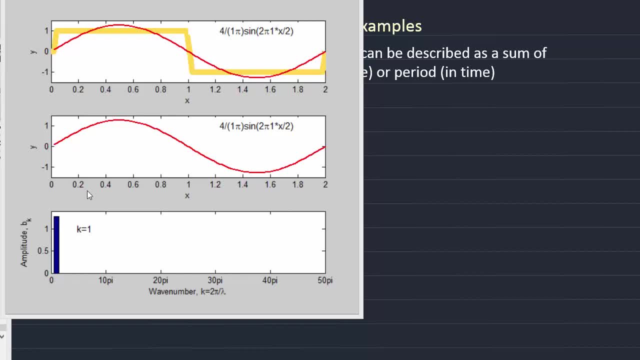 In this case, the first amplitude is a little over 1, as you can see here, And it has a wavenumber which is 2 pi over lambda of 2 pi over 2.. So, in other words, it has a wavenumber of pi. 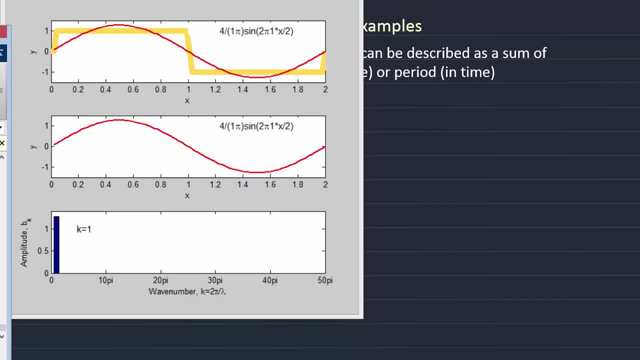 So that's what this vertical bar is. Now let's consider another, a higher wave with a shorter wavelength. This particular wave has a wavelength of a third of the original one, And when we add that function to the first, you can see that we're starting to get a function that starts to 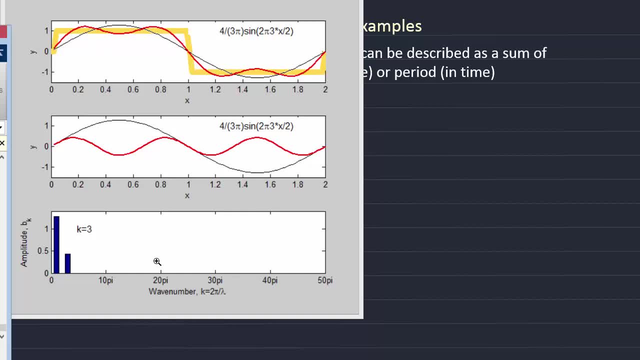 better approximate our original square wave function. This adds another component to our periodogram at a slightly smaller amplitude and greater wavenumber. So as we add successively higher frequency or shorter wavelength signals in, you can see that the resulting signal becomes a closer and closer approximation to the square wave. 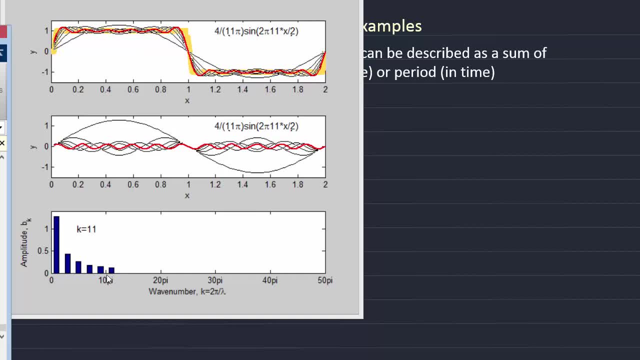 And as we're adding to the total function, we're also adding to our periodogram, And we're adding successive sine functions of higher or shorter wavelength and smaller amplitude, Until eventually we get a function that looks very close to our original square wave function. 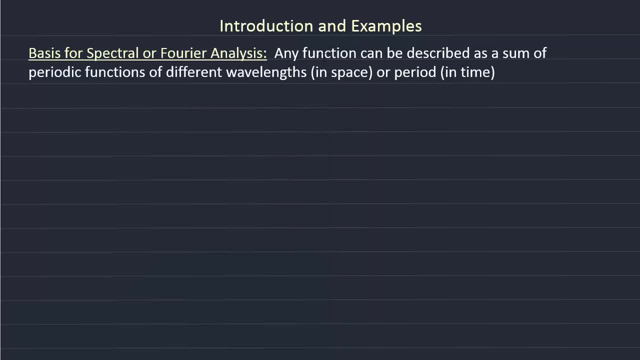 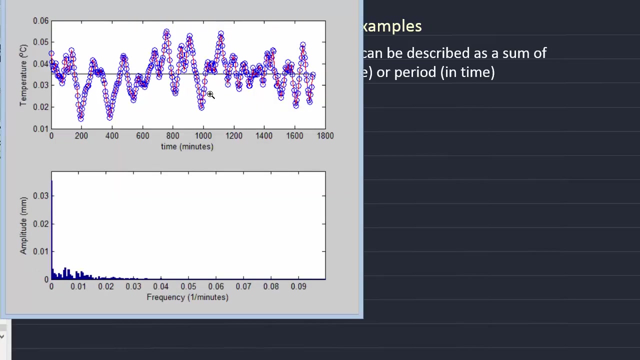 So this illustrates the concept that any function can be described as a sum of periodic functions of different wavelengths. Now another use of this analysis will be illustrated in this example. So let's get this going. So this shows the record of temperature. 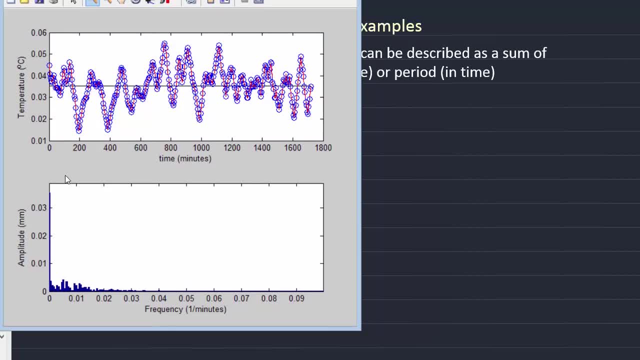 from our last homework problem in a borehole And the temperature fluctuations result. they're caused by fluctuations in water temperature as the water is convecting in the ground at a given depth. Okay, so this is temperature as a function of time, measured at a given depth. 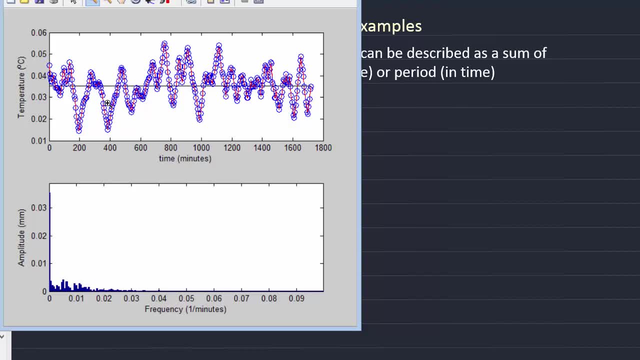 And we did this in our last homework. we used this data set in our last homework assignment to see if there is any strong correlations between this record and itself in an autocorrelation function, And we found that in fact there was a strong correlation. 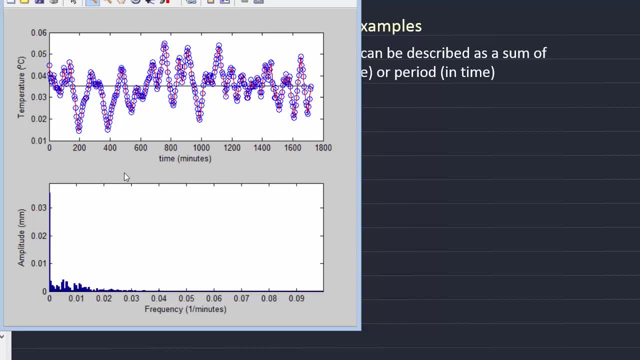 if the record was shifted with itself over about 150 to 200 minutes, suggesting that there was some sort of periodicity in the record over that period of time. So if we do a periodogram of this same record, much like I showed you before, 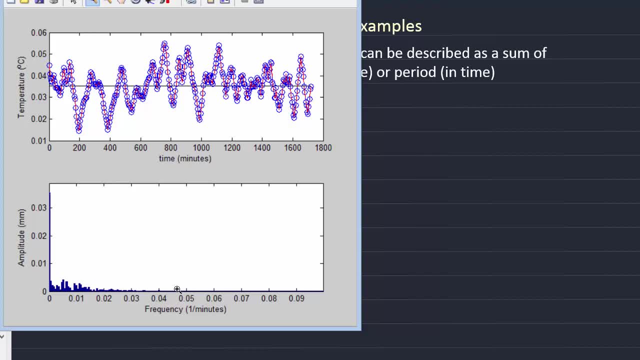 let's zoom in. let's zoom in here a little bit. This is a record of time. so the periodogram I'm showing you here has frequency on the x-axis and the biggest signal occurs at a frequency of zero, and that turns out to be the mean value of the temperature. 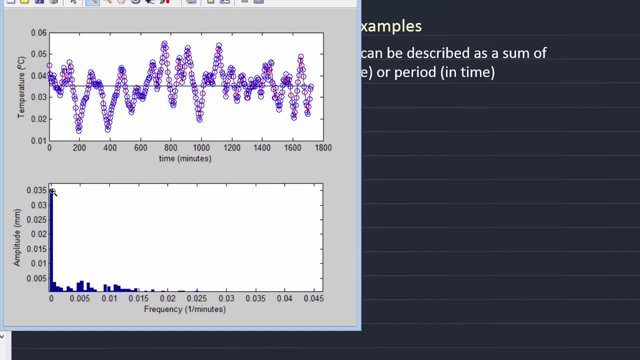 The mean is a little over 0.035, and this shows the value of that mean amplitude. But as we go to actual fluctuations in temperature, you can see that there's a peak near about 0.005, a frequency of 0.005,. 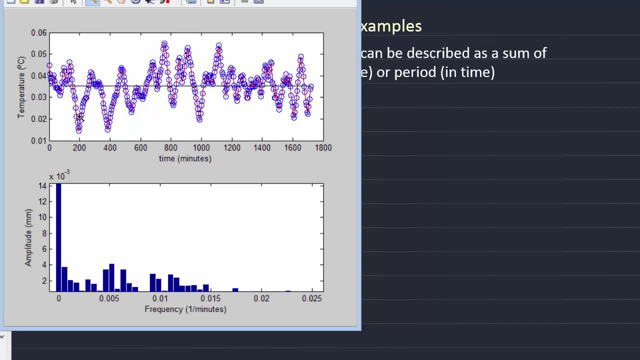 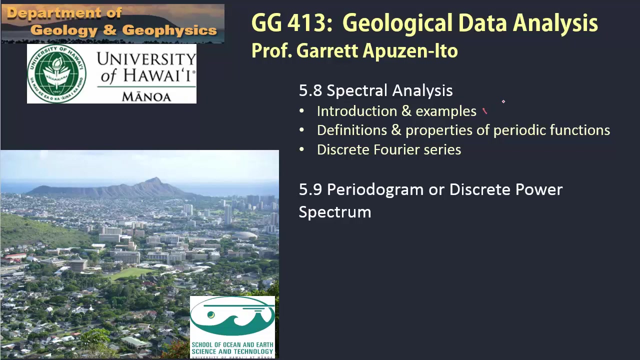 and that corresponds to 200 minutes or so. So this shows that there's a dominant amplitude in the signal with a period of about 200 minutes. So this is a way of identifying some of the dominant periods in a time sequence. So that was our introduction and examples. 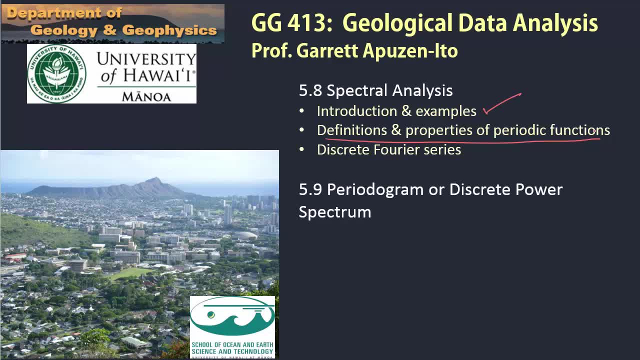 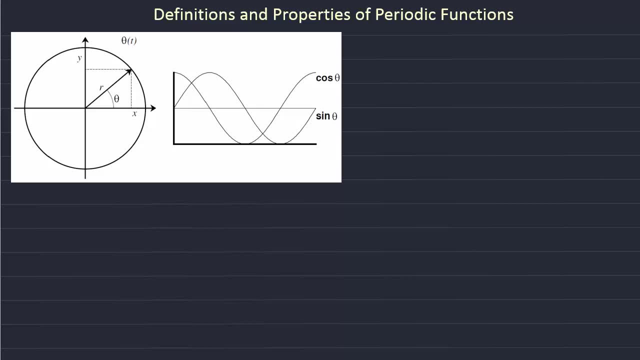 Now let's get on to some definitions and properties of periodic functions. So you've probably learned about sines and cosines in high school, in trigonometry And, as you recall, if you have a unit circle, a circle of radius 1,. 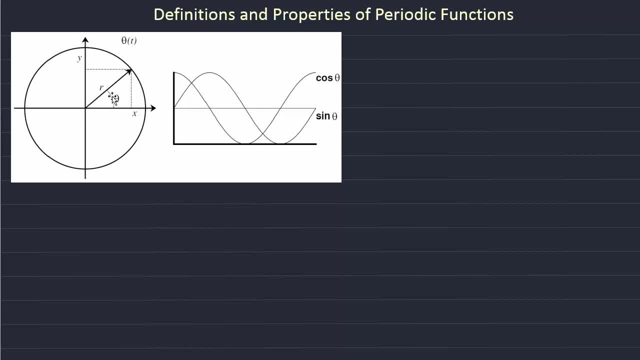 and you draw a line between the origin and to any point on the circle that's our radius vector, then the horizontal component of that vector is cosine of the angle of the radius with the x-axis, So that's cosine theta, And then the y component is sine theta. 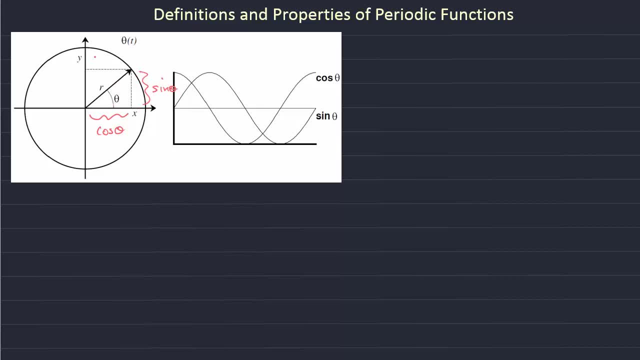 So as we spin this radial arm around the unit circle, and as we do so, as we change theta, then of course the cosine function goes from 1 down to minus 1 and back up to 1.. And likewise the sine function starts off at 0,. 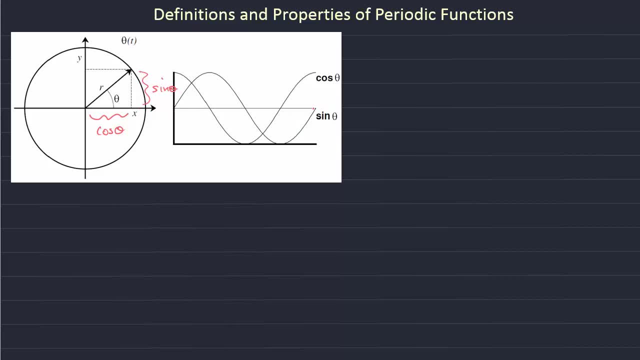 it goes up to 1, down to minus 1, and then back to 0. So we could describe a periodic function as: y equals a cosine theta, And that's an example where a represents the amplitude of the cosine function. For the unit circle, that amplitude is 1,. 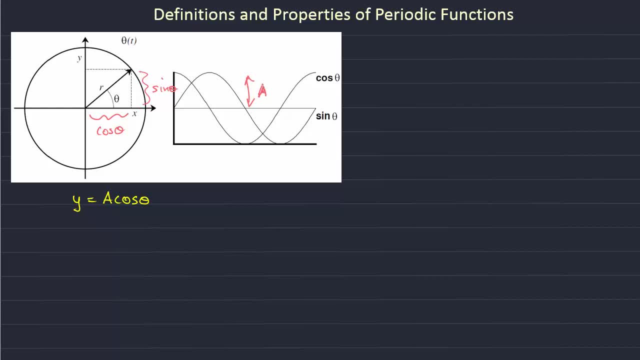 but for a general function, the amplitude could be any number. Now for an oscillation in time. let's look at the cosine function, In other words. another interpretation of this cosine function is: it describes an oscillatory behavior as a function of this horizontal axis. 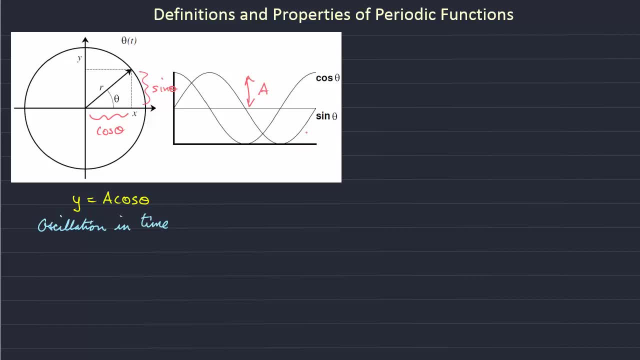 And in the first example the horizontal axis was, of course, theta, but it could also be time, In which case theta would be described as omega times time, where omega is our angular frequency, 2 pi over our period, And we would have: y is equal to. 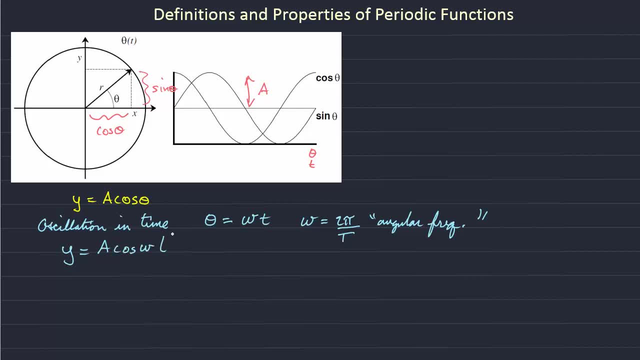 a cosine, omega t, For an oscillation in space. our cosine, the horizontal axis on the above plot, would be, for example, x, representing space, And theta is equal to k times x, where k is equal to 2 pi over the wavelength. 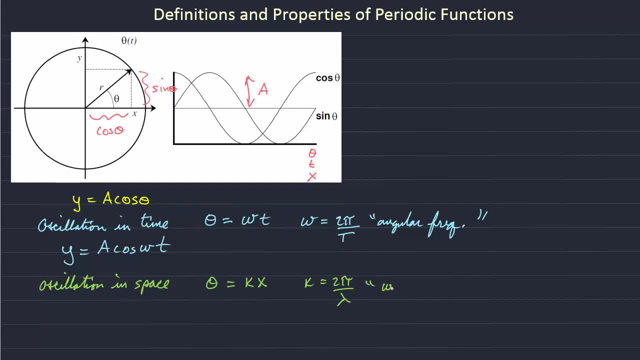 of the oscillation And that's called our wave number, And y would be described as the amplitude times cosine kx. Now following up on the function of an oscillation in time, if omega is angular frequency, then the frequency is just 1 over t. 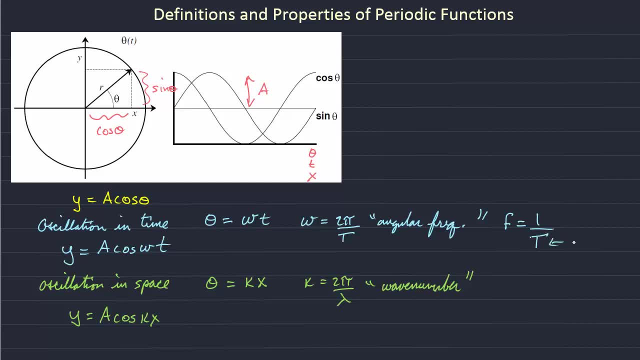 the period. So t is period. So these example periodic functions are of course cosine functions and they start off at the amplitude, at t equals 0. But that's not necessarily a general case, because what defines 0 is arbitrary and the cycle could start at a later time. 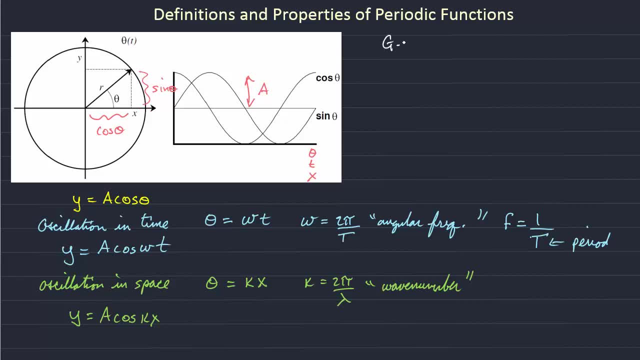 So a general periodic function is described, for example, as a function, again with our amplitude of cosine, and I'll take an example in which it's an oscillation in space, cosine kx minus phi, where phi is a phase shift, or I should just the phase. 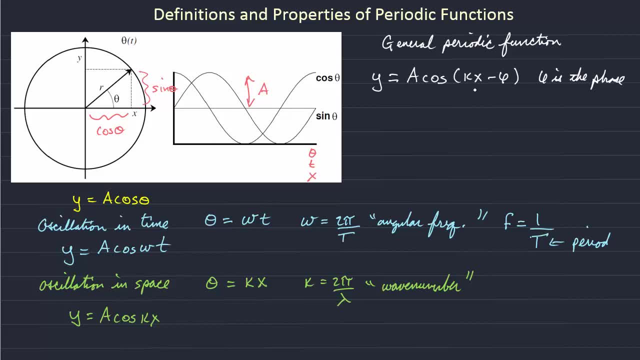 It describes how far off of x equals 0 that the oscillation begins. Now this describes two free parameters for a given wave number. So that's the first one, and then the second one, and then the third one, and then the fourth one. 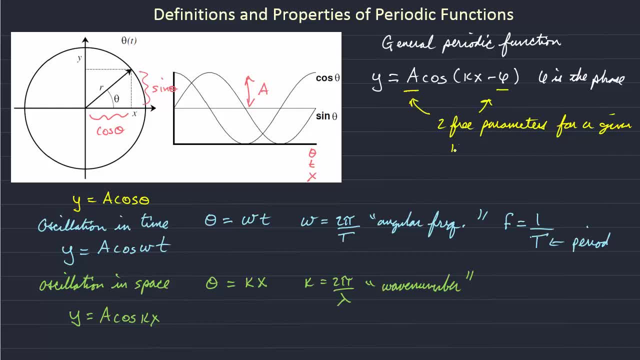 and then the fifth one, and then the sixth one. So this is two parameters for a given wave number that we would, for example, end up solving for when we're trying to decompose an original signal into a superposition of these functions. 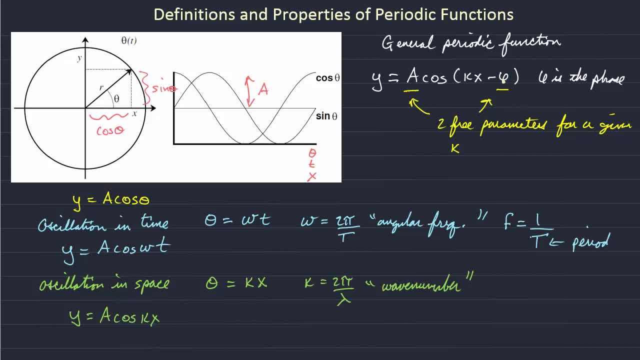 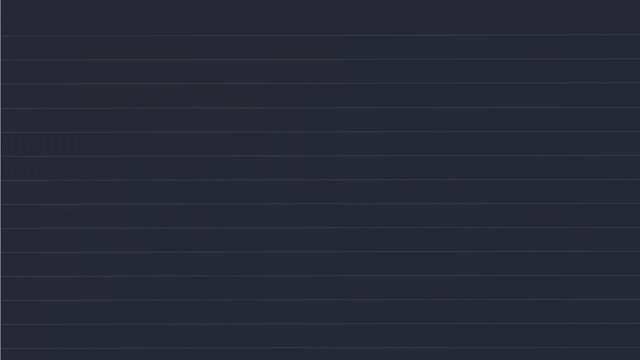 But you'll notice that the phase is non-linearly related to the basis function. It's the argument in the cosine. So describing the general function in this way can be complicated. So it becomes more practical to write this general periodic function in a slightly different form. 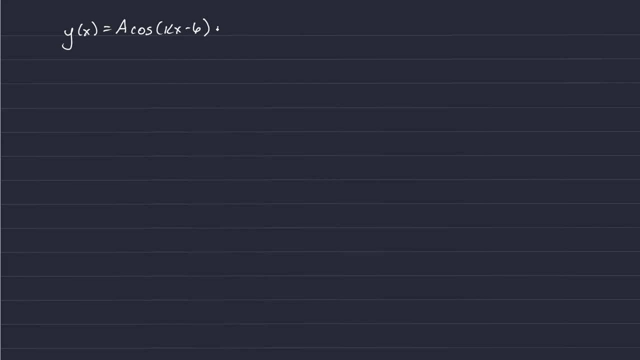 using a trigonometric identity which describes this phase shift instead of in terms of products of other periodic functions. So the first function is a cosine function and it has an amplitude of little a, which is a times cosine function, A times cosine phi. 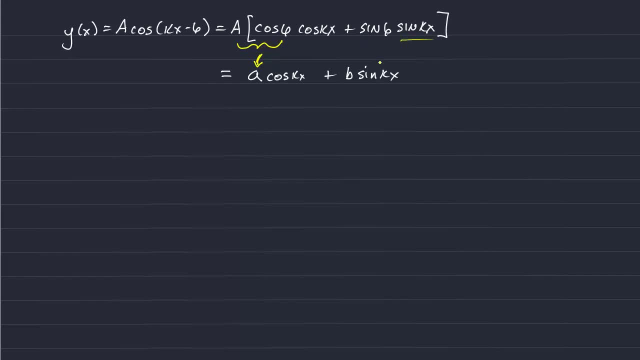 And the second function is a sine function and it has an amplitude of a times sine b. So in this form a and b are now linear functions. They're multiplied by the basis, The basis functions. So now we have a linear relationship. 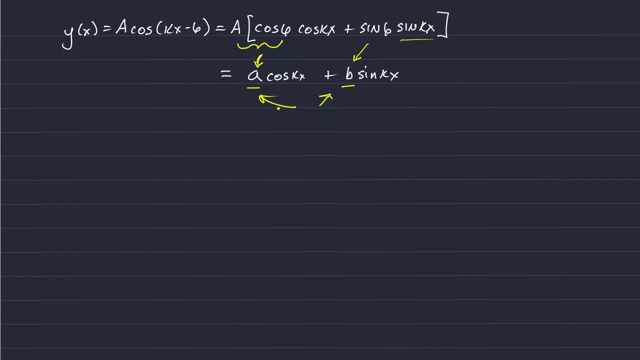 between our two independent, our two parameters describing the function And going, showing the relationship between big A and our two new parameters. Big A is the square root of a squared plus b squared And phi is simply the arc tangent of b over a. 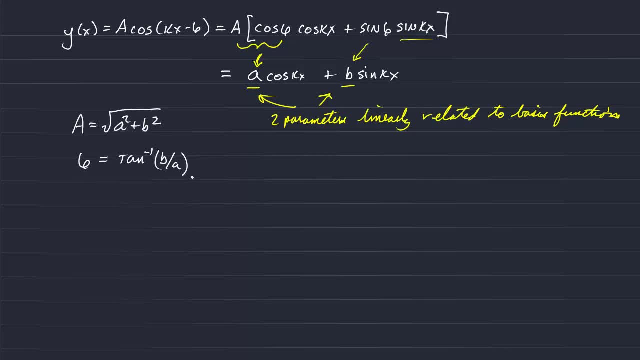 Or tangent of phi is equal to b over a. So we're going to use this function or this form of a periodic function to describe the general periodic function. Now, any real, any true data sequence that we have of course has a finite number of measurements. 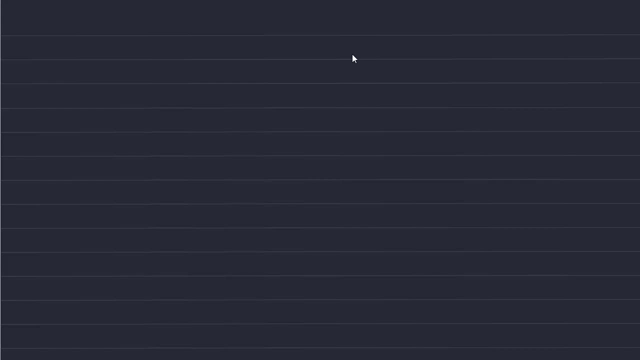 And they're taken at discrete points. Thus this data sequence must be described as a sum of discrete periodic functions. So now we can discuss that: the real number of integers in the final equation and the value of the real number of integers in the final equation. 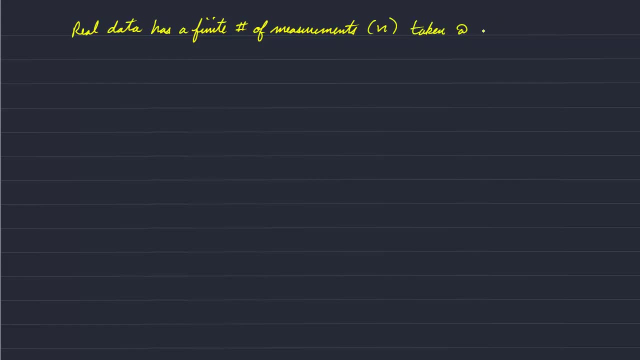 So what's the first number? What's the final number? Well, the last number, you know, is the current number of integers in the final equation. So that's the initial number And then the other number is the number of integers. 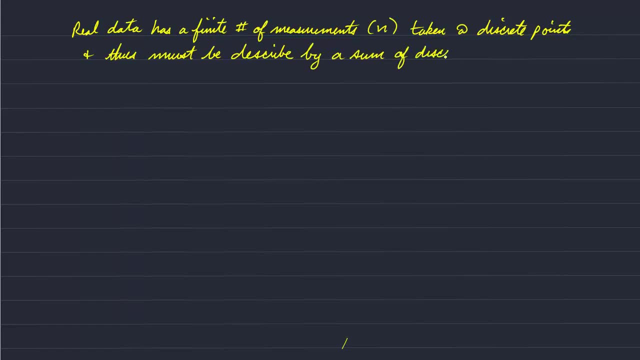 And how many integers is that? So let's define big T as the duration of the whole record. This is our whole data record, the total duration of the whole record. So the first or fundamental frequency that we can resolve with this data set has a period. 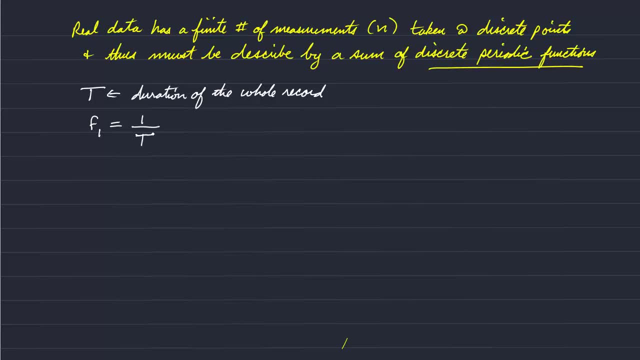 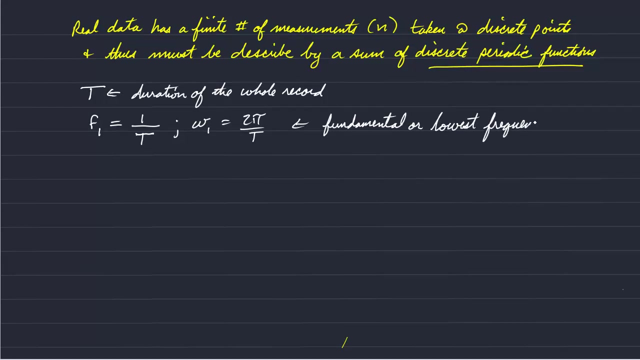 of big T, or frequency of 1 over T, And the fundamental angular frequency is 2 pi over T, And because this oscillation starts and ends with a period of exactly T, it is also called a harmonic. So a harmonic function is a function that starts and ends at the beginning and end of 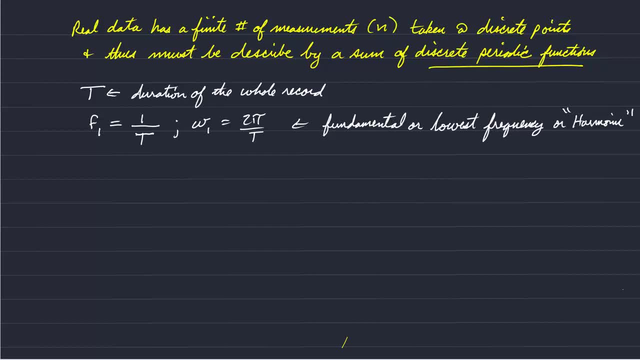 the full record. It has an integer number of oscillations across that period. So the lowest harmonic has a period equal to the length of the entire record. The second harmonic has a period of half the total record length. So this is our second harmonic. 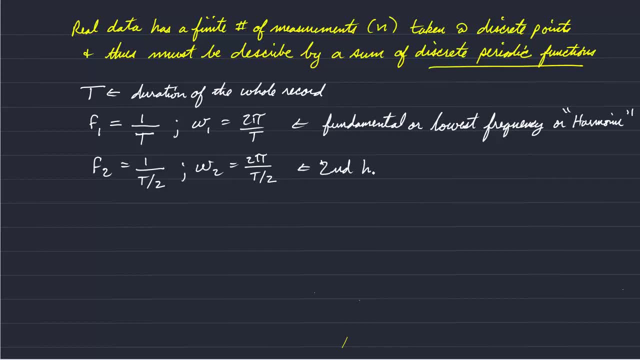 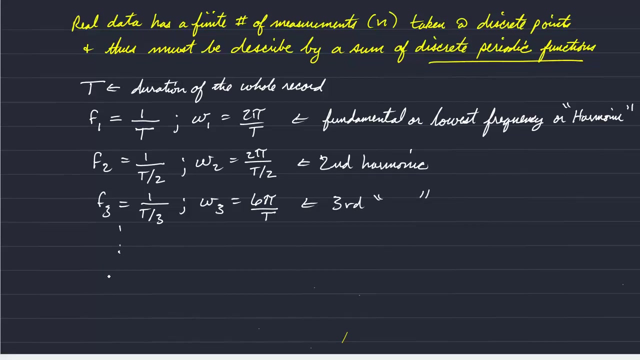 The third harmonic has a period of a third the total record length, and so on, all the way down to our n-2 harmonic. And sorry, yeah, this is our n-divided-by-2 harmonic. So the j-th harmonic. 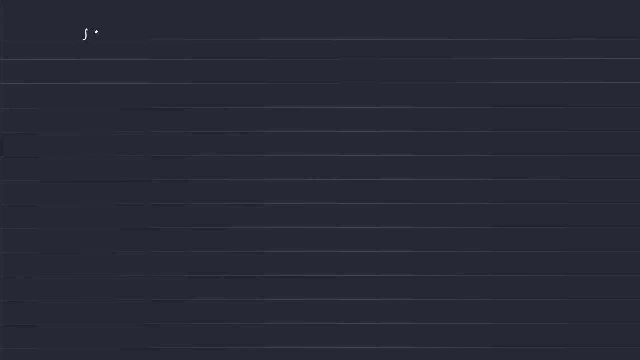 is described as, for example, y is equal to aj cosine omega j, t. So okay, I'll describe what the i's are in just a second: bj sine omega j, t, i. So the j-th harmonic is the n-divided-by-2 harmonic. 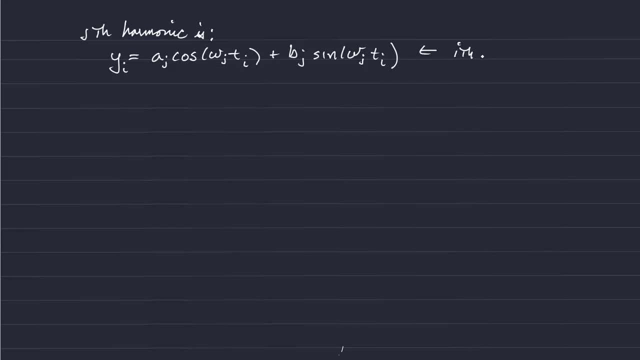 So this is the i-th value of y at time t i for the j-th harmonic, where j describes the frequency of this particular signal. Now t sub i, the time at the i-th point is equal to i times t, i times delta t. 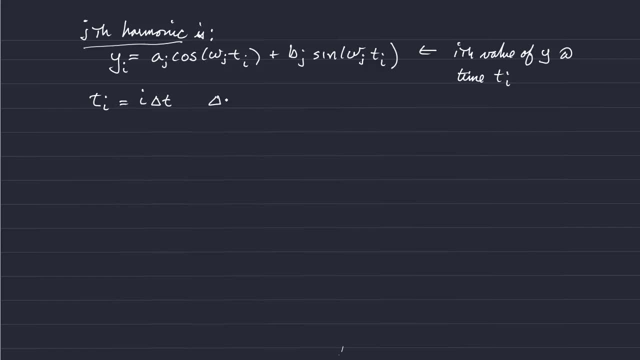 And here we're assuming that delta t is the sample interval, the amount of time between subsequent samples, and it's assumed to be constant. It's constant or uniform across the record. So the i-th sample occurs at t sub i And we can describe wj. 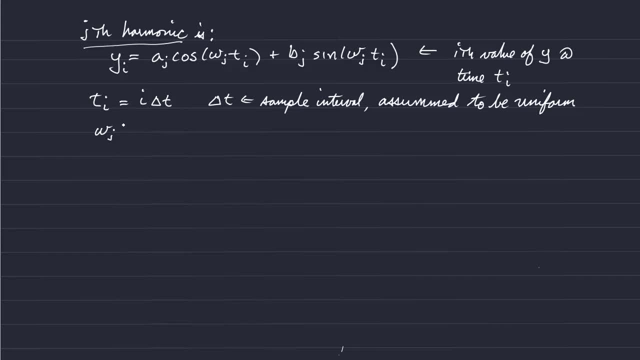 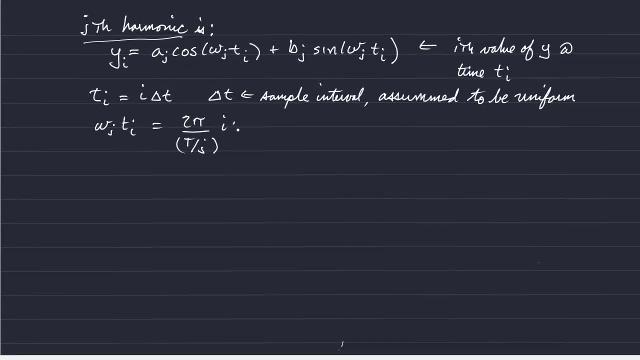 times i delta t times i delta t, and that's equal to 2 pi j over t times i delta t, and that's equal to 2 pi j over n delta little t, deltaatrips and n delta t sorry. 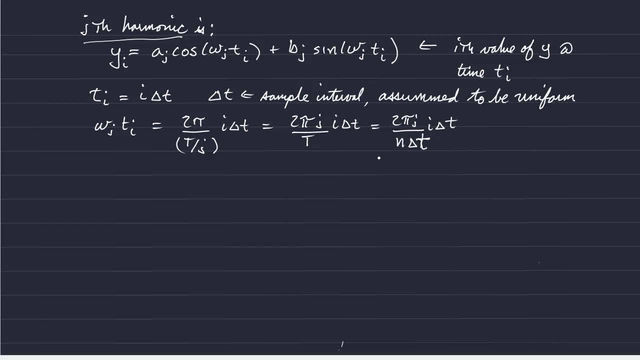 delta little t. delta t And delta t. sorry. delta little t. delta t n. delta t de sb1,6, n. delta t is the length of the whole record because we have n samples separated by the space. delta t: 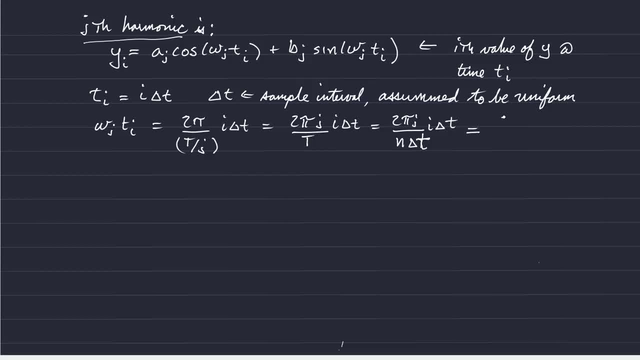 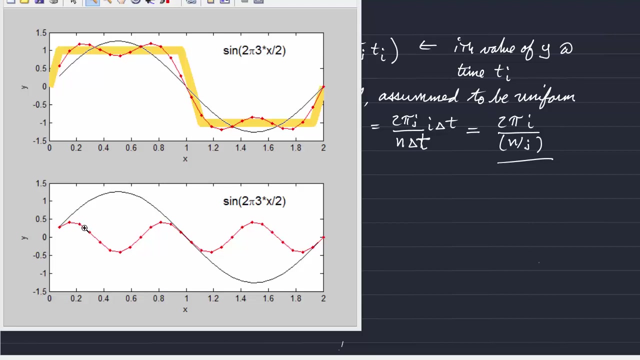 and that's simply equal to 2 pi i all over n divided by j. So these are different ways of writing WJTI in terms of the indices of each record and the total number in the record. So, going back to our example of our square wave, and here I'm looking at the j equals 3 harmonic. 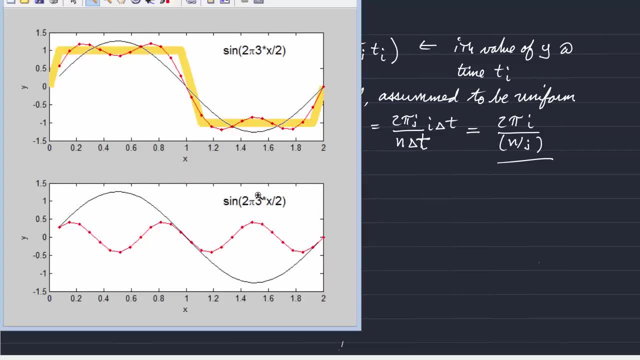 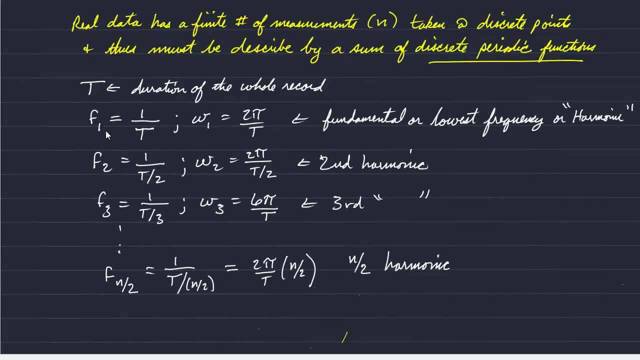 So this is j equals 3.. And I'm plotting dots at each point at which we sampled our square wave. So the time interval between each dot is, of course, delta t, and this shows y at each ith point of this particular harmonic. And again, the lowest frequency that we can describe by our record. 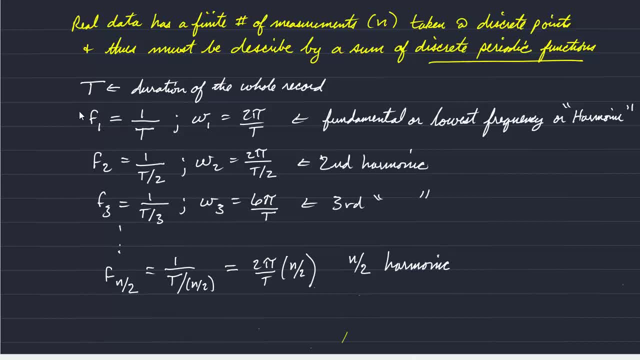 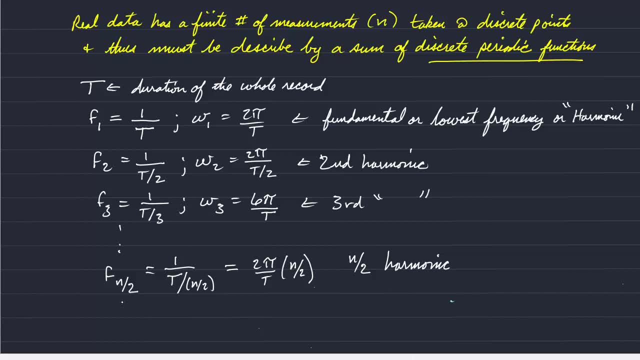 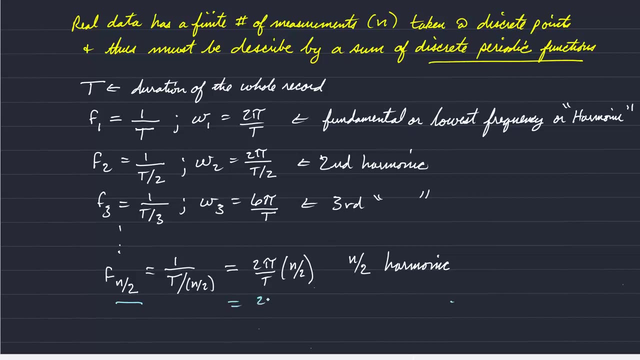 has a period of 1 over t. Our lowest frequency is our fundamental frequency And the highest frequency resolved that we can resolve is described by our n over 2 harmonic. So let's write this big T out in terms of little delta t. 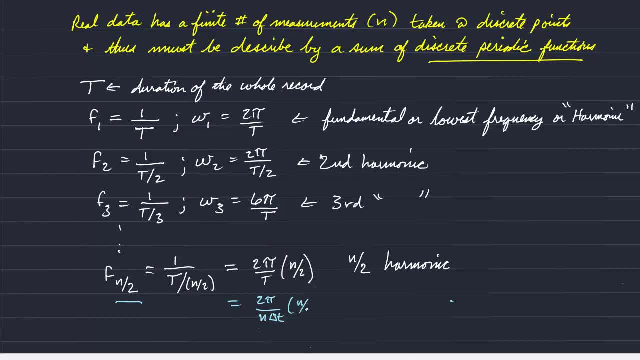 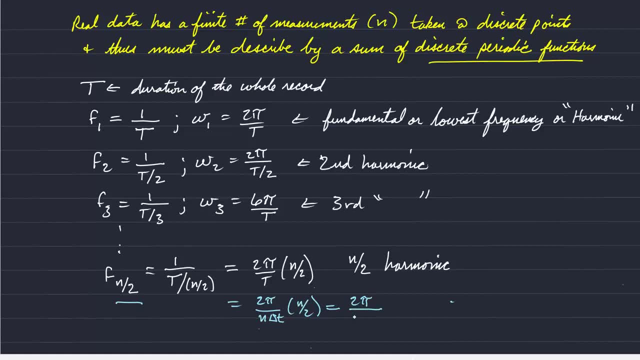 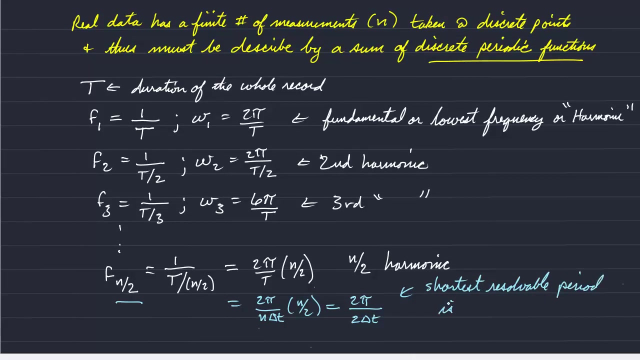 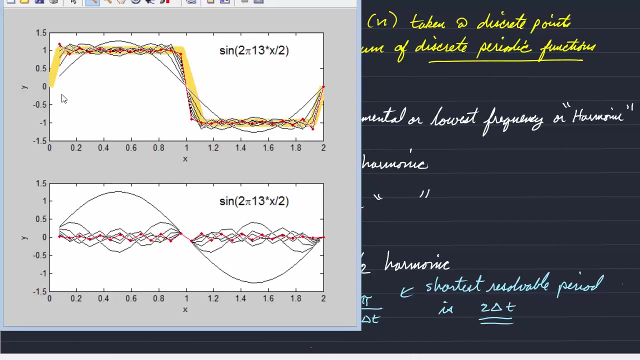 which is again our sample interval, And you can see that the shortest period that we can resolve has a period of twice our sample interval. So let's look at what that shortest period is in our decomposition of our square wave. So this red line curve here represents the highest harmonic that we can resolve by this particular sampling. 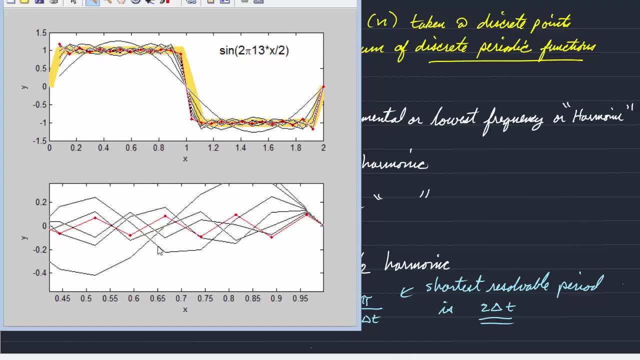 And you can see it, zigzags between each sample interval. Our sample interval here is about 0.07 or something like that, But you can see that the shortest period we can resolve is is a period of 2 times the sample interval. 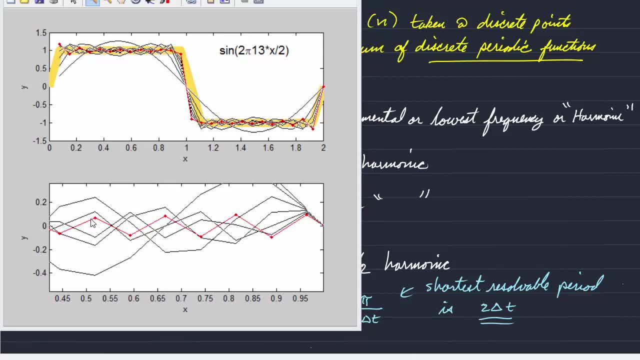 This is a very crude representation of a cosine function that starts off at 1,, goes to minus 1, and then back out over 1, over twice the sample interval. So that's an illustration of why our shortest period is 2 times delta t. 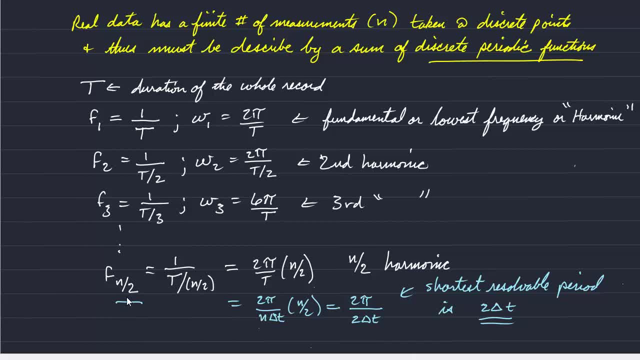 It turns out that the highest frequency is called our Nyquist frequency, So our sample interval is 1.07.. Just describing some terminology that you'll see coming up in harmonic analysis. So it looks like I'm running a little bit out of time for this particular video. so I'm going to stop here.